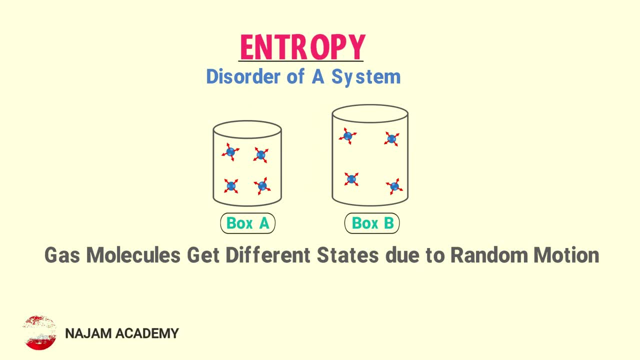 this important statement. Over time the gas molecule both in box A and box B get different stats due to random motion. Now the gas molecules in box A are moving freely in a small space compared to gas molecules in box B. In physics we say that over time, due to less available space in box A, the gas molecules will. 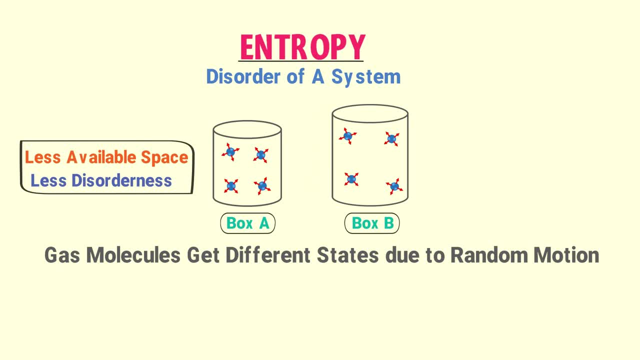 get less disorderness, while here in box B we say that over time, due to large available space, the gas molecules will get more disorderness. Simply remember that gas molecules are moving freely in a small space compared to gas molecules in box B. Thus I say that system of box A or system A is less disorder, while system of box B or system B is more disorder. System A is less disorder and system A has less entropy. System B is more disorder and system B has less entropy. 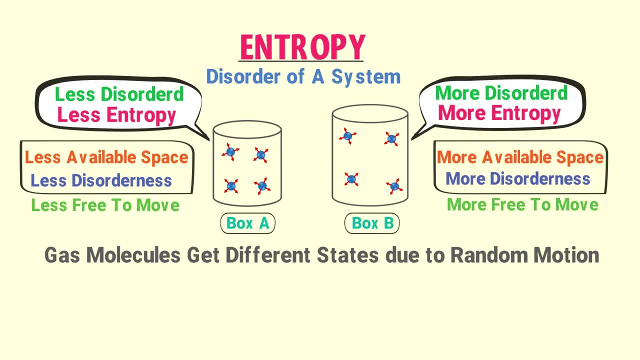 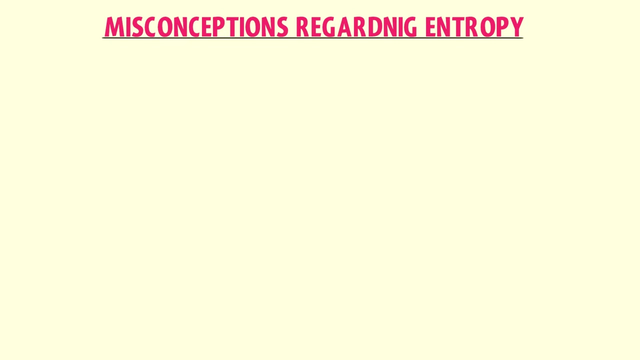 has more entropy. Thus, from this example, we learn that over time, due to external factors, the state of gas molecules changes. Hence the state of gas molecules changes, entropy changes. Now let me clear the common misconception regarding entropy. You often read or learn that people relate entropy with clean and 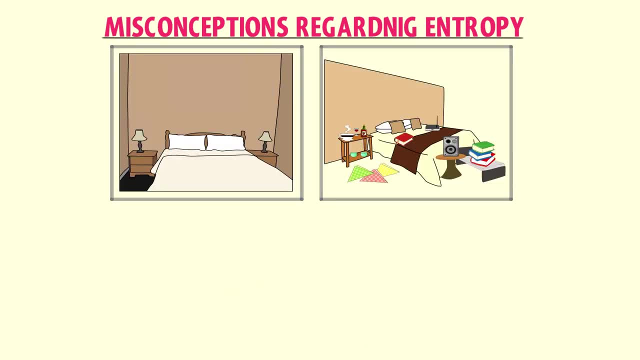 dirty room. They say that people relate entropy with clean and dirty room. They say that clean room is more ordered, while dirty room is more disordered. Thus clean room has less entropy and dirty room, due to more disorderness, has more entropy. But this is wrong example. Let me explain. 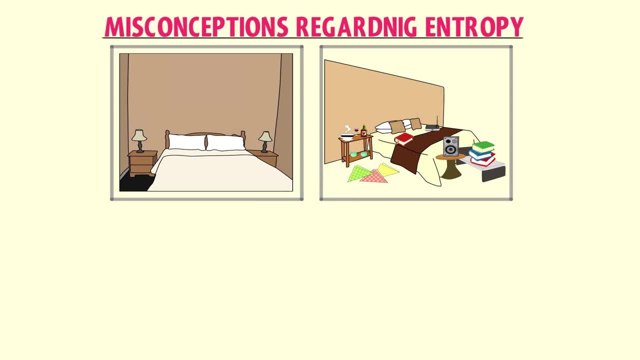 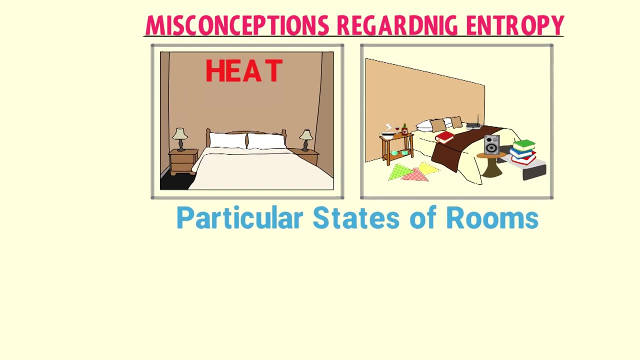 it The first thing you should know about this example that it is the particular state of these rooms. Let consider that you add some amount of heat to this clean room by putting heater in it. This addition of heat would increase the kinetic energy of gas molecules and the clean room. They 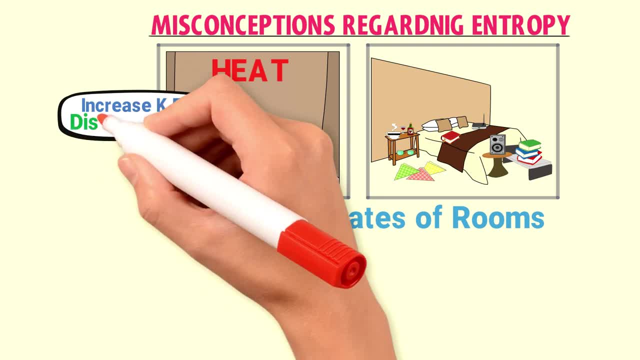 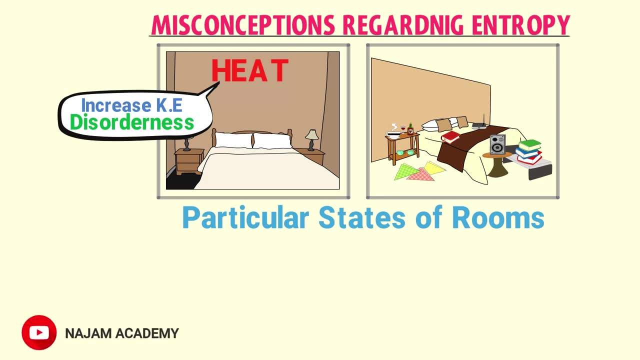 will start moving with greater speed, Hence the disorderness of gas molecules and disorderness of all the stuffs, and the room would be large. Thus this clear room will have more entropy than this dirty room. Now the correct example is that you are angry and you enter to. 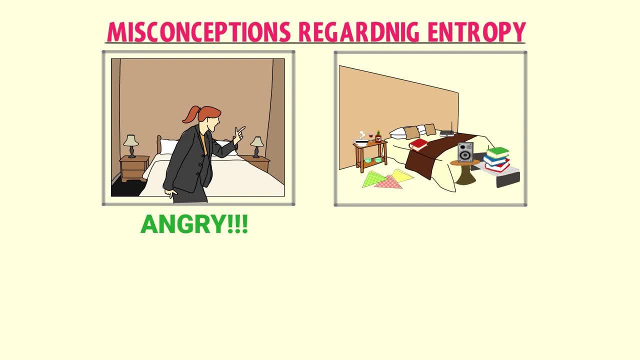 this clean room, You started throwing all the things in the room here and there. Thus you changed the order of this clean room, You changed the entropy of this clean room. Similarly, if you enter to this dirty room, happily, you just keep everything on its respect. 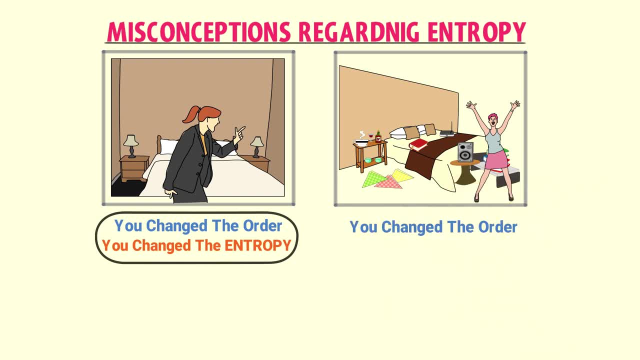 position. thus you change the order of this dirty room, you change the entropy of this dirty room. thus, remember that entropy doesn't depend only it one particular picture or absolute state of an object, or anything, but over time the state of the system changes due to many factor. thus entropy also changes. now let 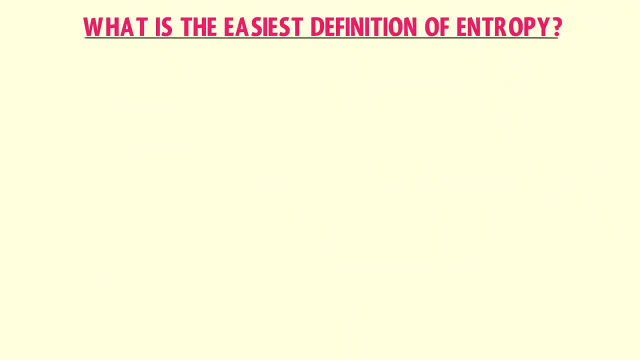 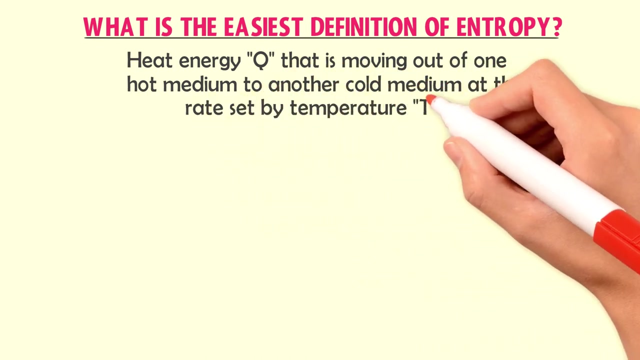 me teach you that. what is the easiest definition of entropy? personally, I define entropy as the heat energy Q that is moving out of one hot medium and to another cold medium at the rate set by temperature T. the second standard definition of entropy is the unavailable or unusable energy within a closed or 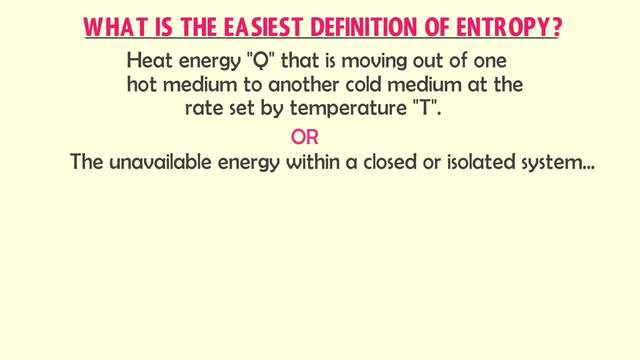 isolated system is non-existent as a entropy. Here let me clear the term unavailable energy or unusable energy, or why we call entropy as unavailable energy. The answer is very simple. We dissolve sugar or salt and water. Chemical bonds among the sugar or salt molecules break down. The sugar molecules are salt molecules. 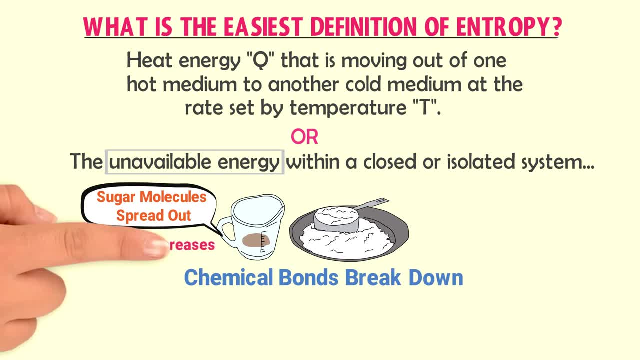 spread out and water. As a result, entropy of system increases due to disorderness of sugar or salt molecules. Now here is the important point: Can you and I use or utilize the energy released during bond breaking of sugar or salt molecules? The answer is absolute: no. 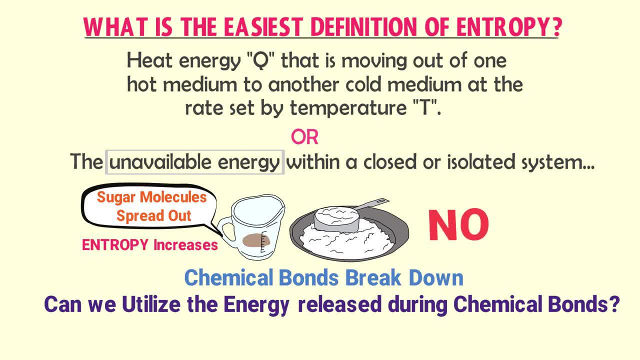 We cannot utilize or use this energy. This energy just improves the quality of the energy and the quality of the sugar increased the disorderness of system. Hence we call this energy as unavailable energy. Therefore it is unavailable energy which increases the entropy of a system. 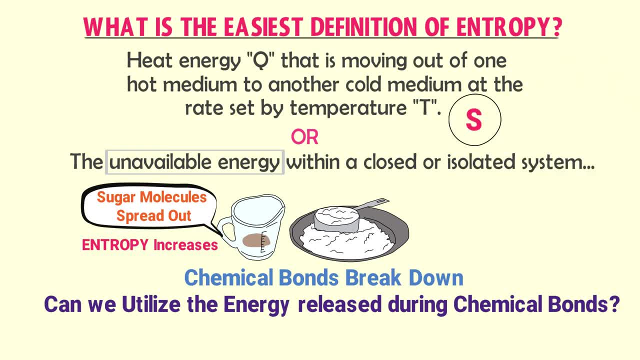 Entropy is denoted by S. The formula of entropy is: S is equal to Q upon T, where Q is the heat added or taken off to or from the system, temperature T. According to my personal experience, students do not have clear concept about entropy. It. 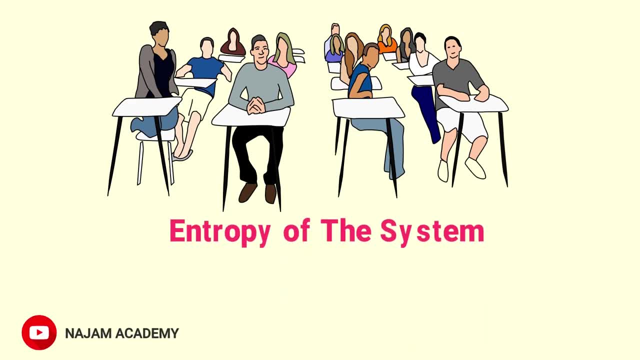 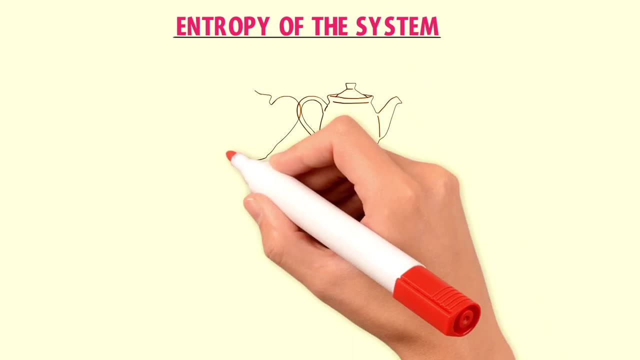 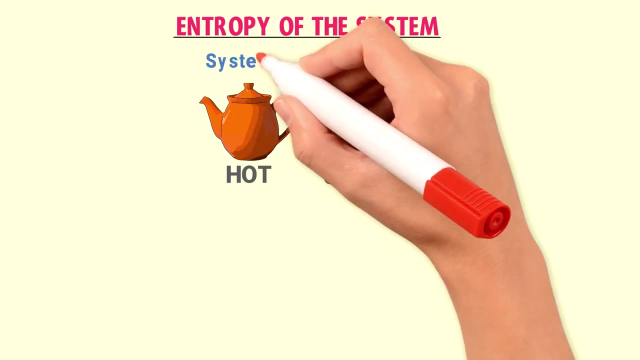 is because they do not understand entropy of the system and entropy of the universe. Thus, let me firstly teach you entropy of the system and entropy of the universe, Hence entropy of the system. Let consider two objects: hot object and cold object. Let I call this hot object a system. 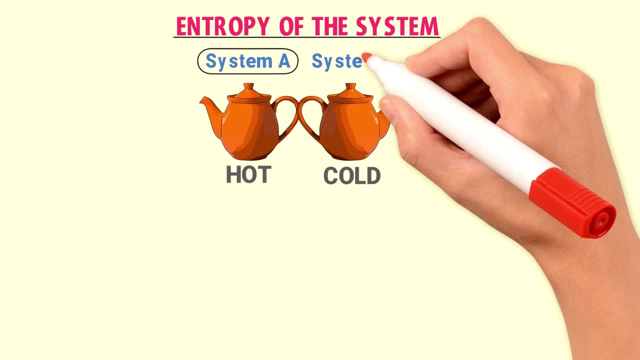 A and I call this cold object a system B. We have learned in one of our previous lectures that heat energy always transfers from hot object and cold object until both the objects get equal temperature and this stat is known as a thermal equilibrium. We know that system. 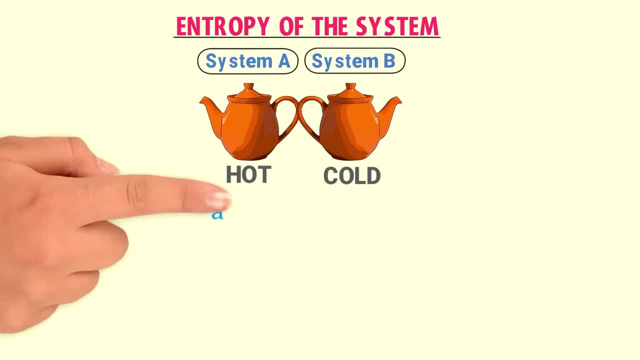 A is hot, hence let its temperature is T A, while system B is cold, hence its temperature is T B. We know that temperature A is greater than temperature B. Now, as a result, a natural process of heat transfer will occur between this hot object and cold object. 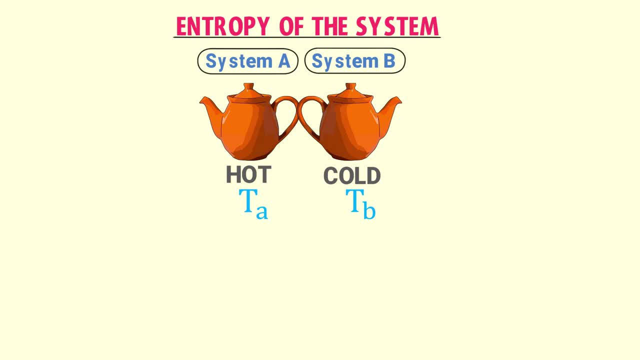 Let this hot object- a system A- losses heat Q. This cold object- a system B- will gain this heat Q. Here remember that heat loss Q by system A is equal to the heat gain by system B. That is why I write single Q for the heat transfer. 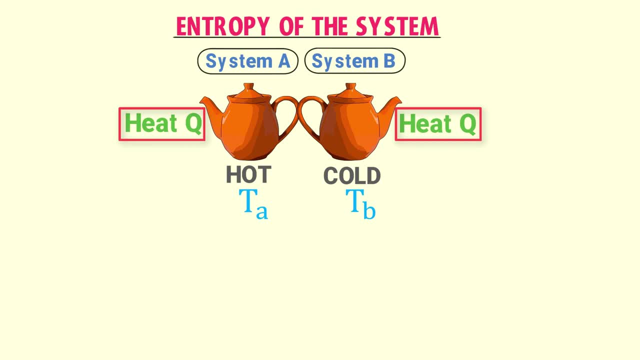 Now here is the most important concept which a lot of people do not learn. Let me teach you Let. the entropy of system A is S A and the entropy of system B is S B. Here, system A losses heat Q. According to physics convention, heat loss is considered negative. Hence system. 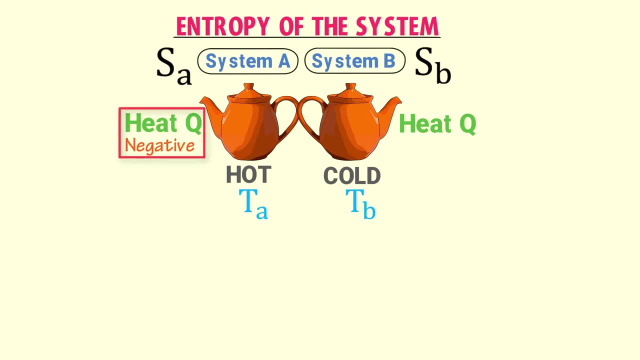 A has lost heat Q. System B gains heat. Heat gain is considered positive. Hence system B has gained heat Q. We know that entropy S is equal to Q upon T. The entropy of system A is S. A is equal to negative Q upon T A, while the entropy of system B is S is equal to positive Q upon T B. It means 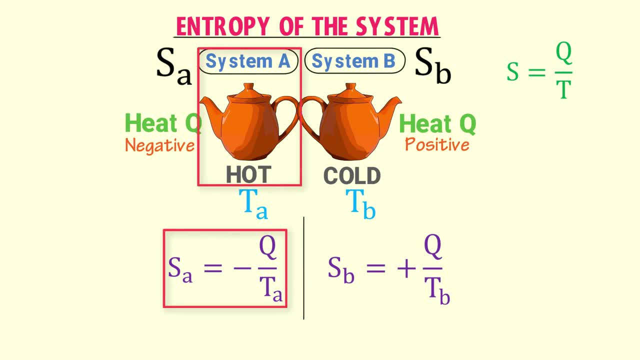 that the entropy S A of system A decreased, while the entropy of system B increased. Thus, from this example we learn that, at system level, if an object loses heat Q, its entropy S decreases or its entropy S is negative. Secondly, at system level, if an object gains, 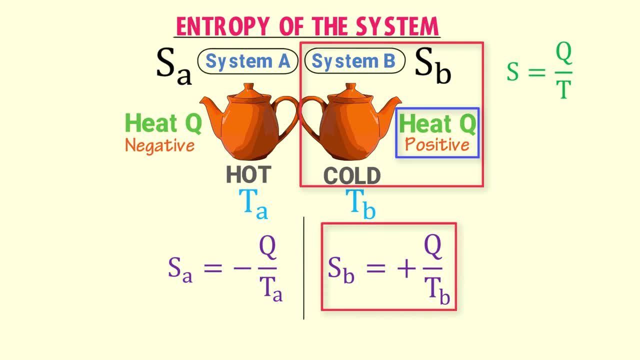 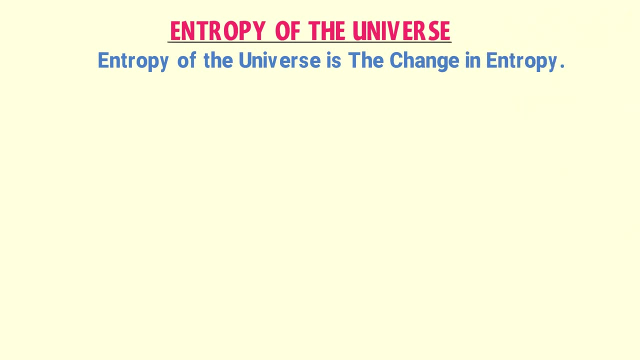 heat Q, its entropy S increases or its entropy S is positive. Note down these important points. Now let me teach you how to solve this problem. The concept of entropy of the universe: Remember that entropy of the universe is the change in entropy. Dallas, Or to measure, or to learn the entropy of the universe, we must measure. 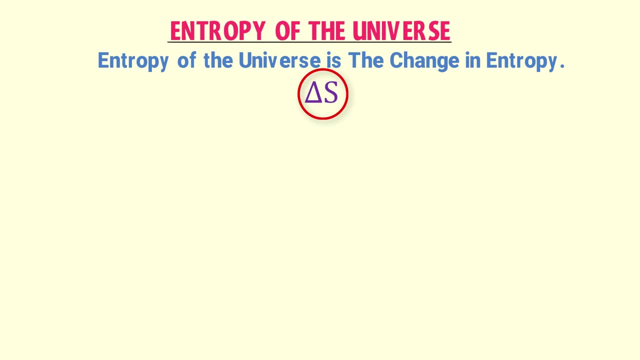 the change in entropy. I will give you 2 cases which will clear your concepts. Case number 1.. Let again consider a cold and a hot object. We have learnt that heat Q will transfer from hot object to cold Q to the cold object. let the initial temperature of hot object is T, 1 is. 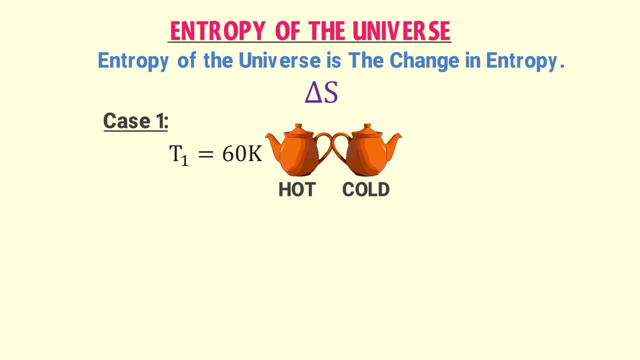 equal to 60 Kelvin and the initial temperature of cold object is T 2 is equal to 30 Kelvin. let hot object losses heat Q is equal to 300 joule and cold object will gain the same heat. Q is equal to 300 joule. now we consider these. 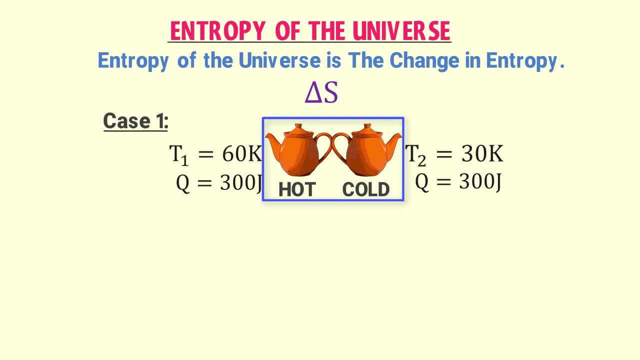 two objects as a universe are surrounding sounds crazy, but this is how physics is learn. now I am interested to find the change and entropy Dallas in these two objects are and this universe of two objects. we know that the entropy of this hot object decreased due to heat loss, while the entropy of this cold object increased due to heat. 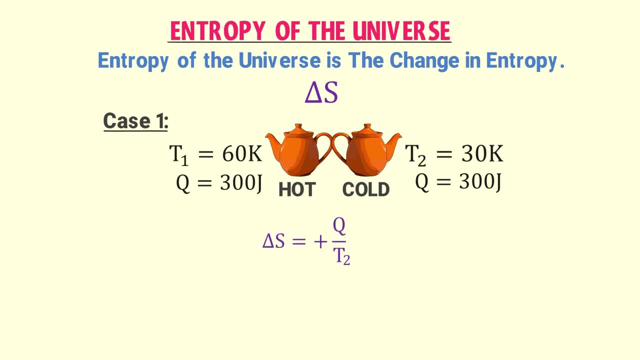 gain. now, Del S is equal to this cold system gained heat Q. hence its entropy is positive Q upon its initial temperature- T 2, while the entropy of this hot system is negative Q upon its initial temperature- T 1. we know that initial temperature of the hot object is T 1 and the entropy of the hot object is 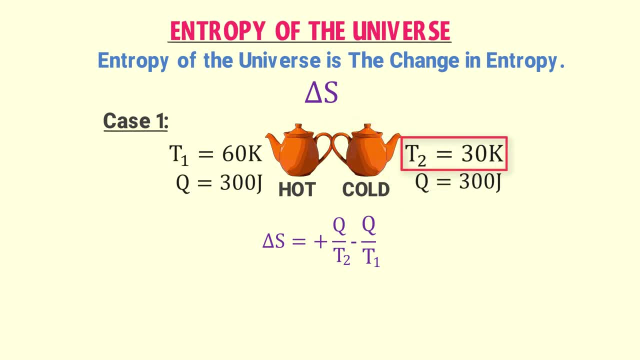 temperature of cold object is T2 and it is equal to 30 Kelvin. We also know that this cold object gained heat. Q is equal to 300 joule. Thus del S is equal to 300 joule upon 30 Kelvin minus. hot object losses heat Q is equal to 300 joule and its initial temperature 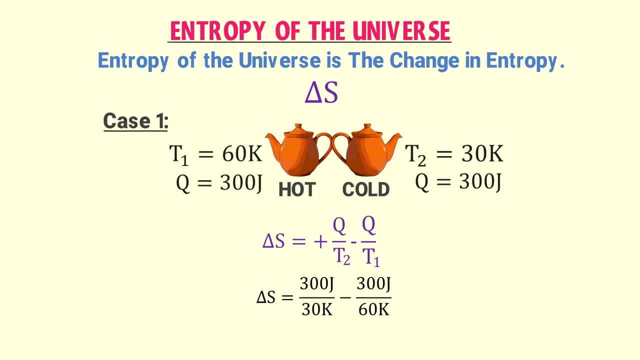 Q is equal to 60 Kelvin, We get del S is equal to 10 joule per Kelvin, minus 5 joule per Kelvin. As a result, we get del S is equal to 5 joule per Kelvin. Thus, this 5 joule per Kelvin. 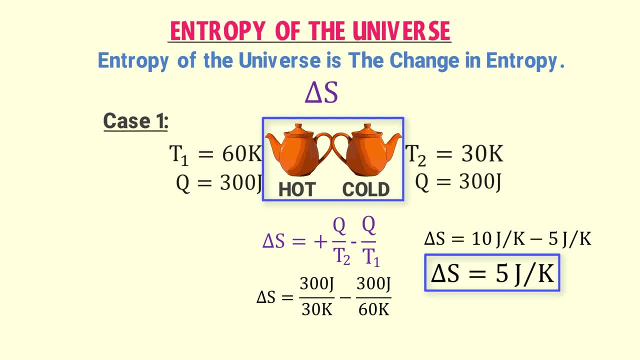 means that the change in entropy is positive. Therefore, first case, that entropy of the universe always increases. Let me repeat this important statement: Entropy of the universe always increases. Thus the total change in entropy and the universe will always be positive. 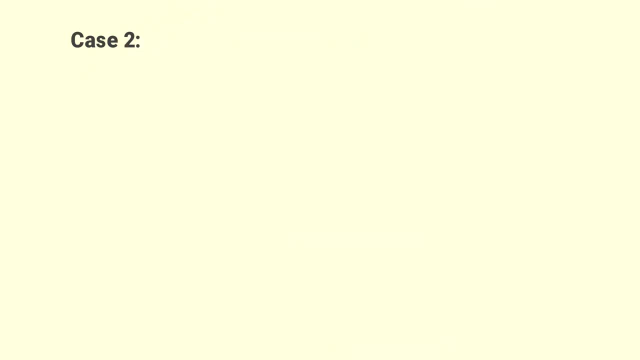 Now let me teach you the second case, or case number 2.. Adiabatic process or reversible process. Adiabatic process is one in which no heat enters or leaves the system. Adiabatic process is one in which no heat enters or leaves the system.